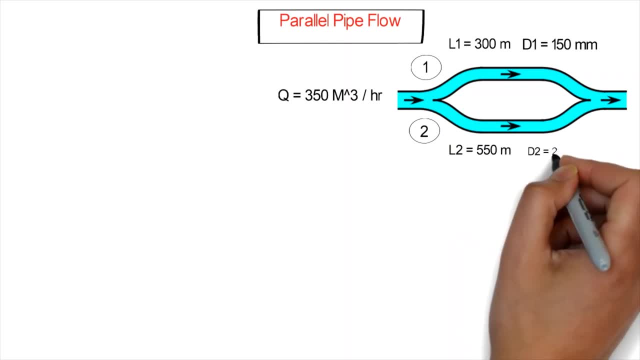 pipe 1 with length equals to 300 meters and diameter equals to 150 millimeter. Also, we have a pipe 2 which length equals to 550 meters and diameter equals to 170 millimeters, and required is and q1 or a is required. so, guys, before we starting solve this problem, we have to discuss something about. 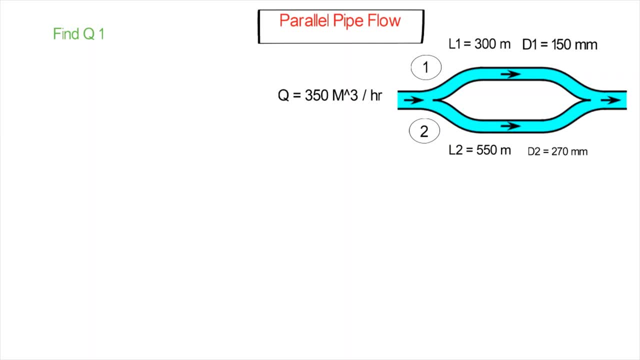 parallel pipe system. we have two essential assumptions here for any parallel pipe system. here in the parallel pipe systems we have the total amount of flow rate or DC charge equals to DC charge in the pipe 1 plus the DC charge in pipe 2, according to conservation. 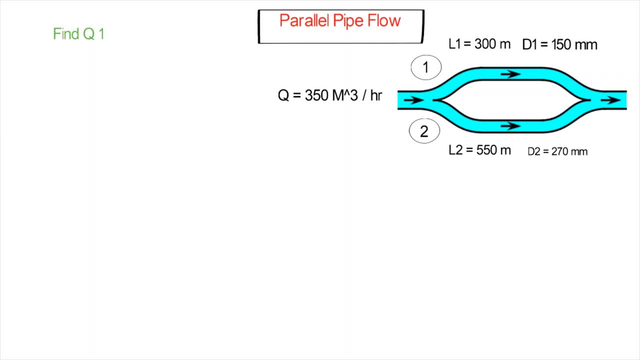 of mass. no, the second one, or the second assumption here, for the also parallel pipe systems, the head losses are equals in each pipe in the parallel pipe system. so, guys, the head losses are equals in each pipe. that's because if you look at the value of total head losses, it will be the difference between 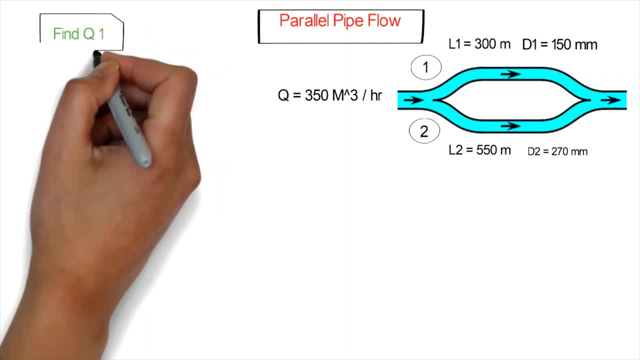 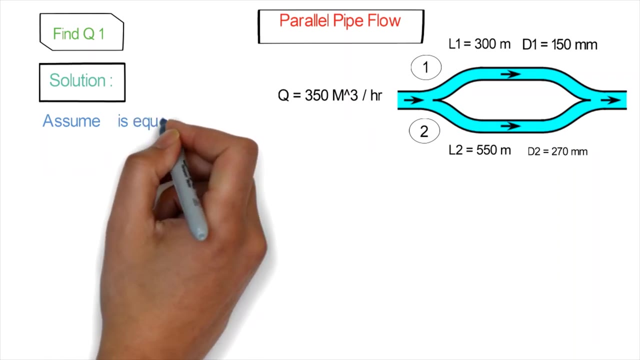 the pressure or the total pressure in the outlet minus total pressure in inlet, and that's because we need one value of pressure in the outlet point. it's not allowed to obtain two values at the end at the outlet point, so your calculations will depend on the output point. 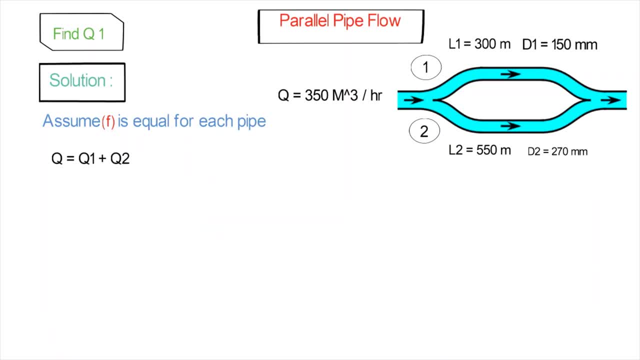 on one value of pressure at the outlet point. it's not allowed to be two values. that's reason why the head losses are equals in each. here we have equation 1: Q equals Q, 1 plus Q 2, according to cool, to conservation of mass. and also we have 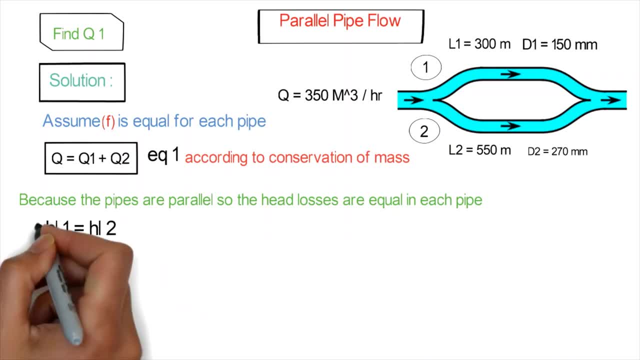 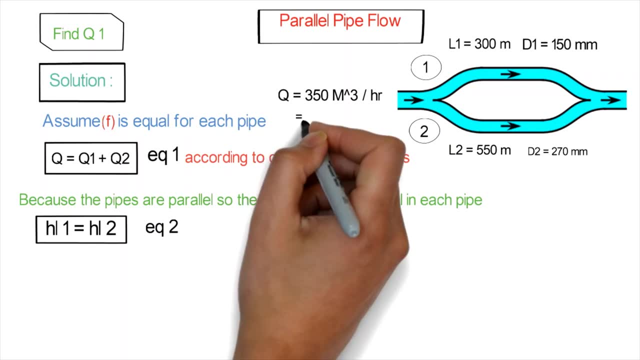 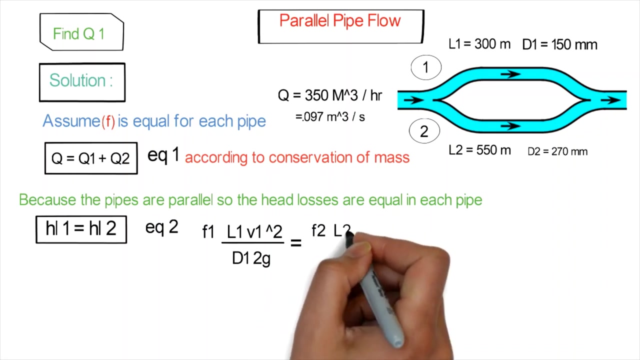 price in pleasing the identified fate llevar. according to Dorothy equation, we have Y F2 times L2 times V2 squared, divided by D2 times 2G. 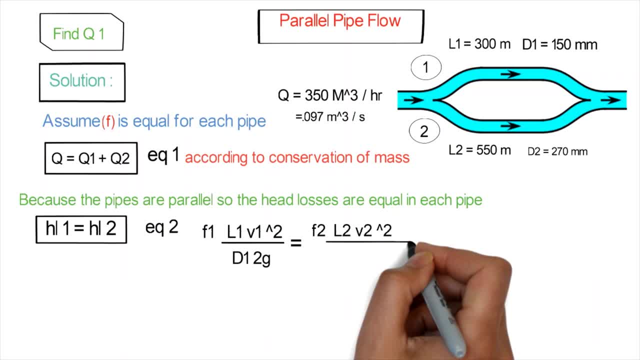 So we have to assume F1 equals F2.. So the fraction coefficient for pi 1 equals the fraction coefficient of pi 2.. So F1 cancels F2 and 2G cancels 2G also. Also, as you know, Q, or the flow rate, equals to V times A, which is V, the velocity and AD cross-section area of the pipe. 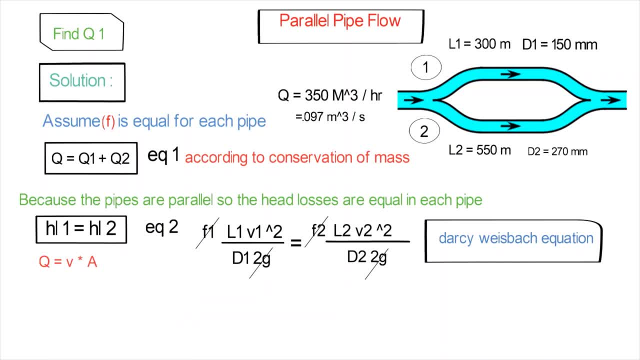 Also the A1 equals 0.017 meters squared, A2 equals 2.057 meters squared, Substitute in the equation 1.. So 0.097 equals to 0.017 V1 plus 0.057 V2.. 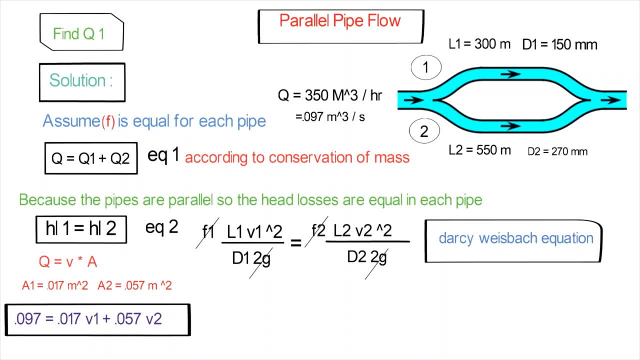